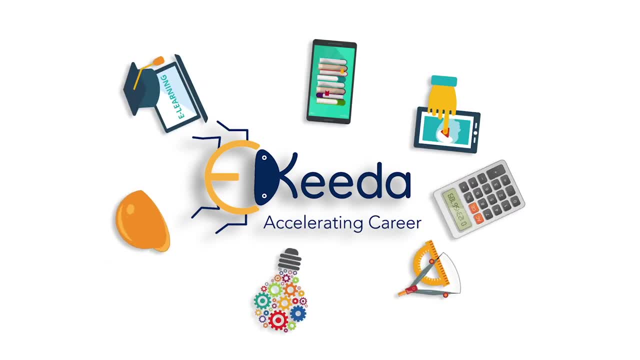 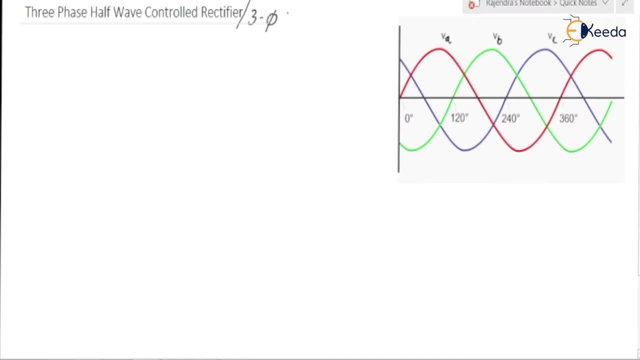 Okay. Okay, so three-phase three-pulse SCR. Three-phase three-pulse SCR. Okay Here, three-phase three-pulse because corresponding to one input cycle in the output. yes, we will be getting the three pulses. That is why it is known as the three-phase three-pulse SC. 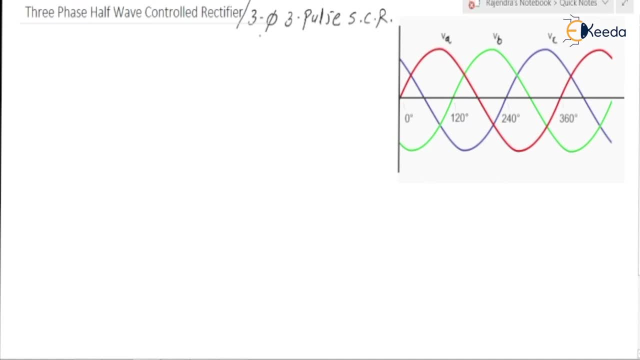 Okay, So important to note: if the input supply frequency is 50 hertz, then the output pulse frequency it will be equal to 3 into 50.. That is a 150.. Okay, So that is why three-phase, three-pulse SCR. 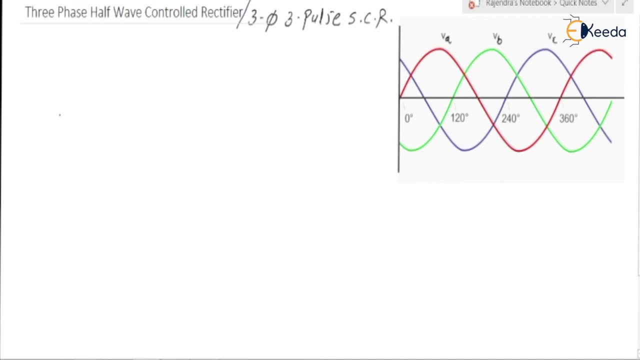 Okay Next. So let us first of all draw the circuit diagram Right. It consists of a three-phase transformer, Right, The primary winding of the transformer. it may be star connected or it may be a delta connected. Okay, So let us consider it is connected in star. 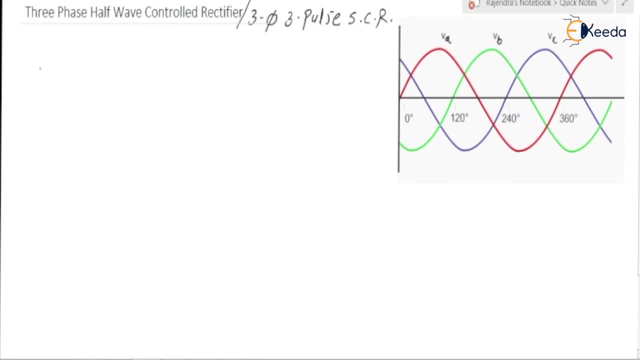 Okay. So here we are having the primary winding of the transformer Right- It may be star connected or delta connected- And the secondary winding Right. Be careful, The secondary winding should be connected in star only. So because here in the three-phase, three-pulse SCR we require a three-phase four-wire supply. 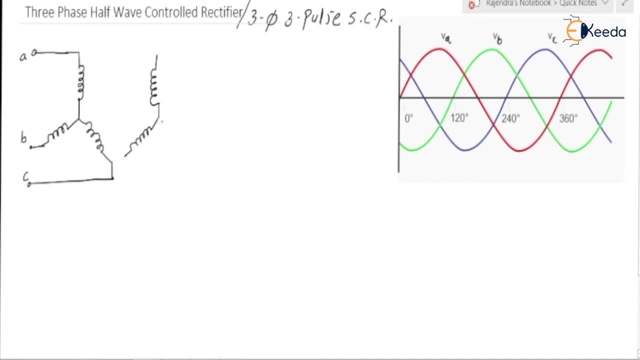 Right Three-phase four-wire supply. That is why the secondary of the transformer should be connected in star, only Right. It consists of three SCRs. It consists of three SCRs: Here it is the first SCR, next second SCR and here it is the third SCR. 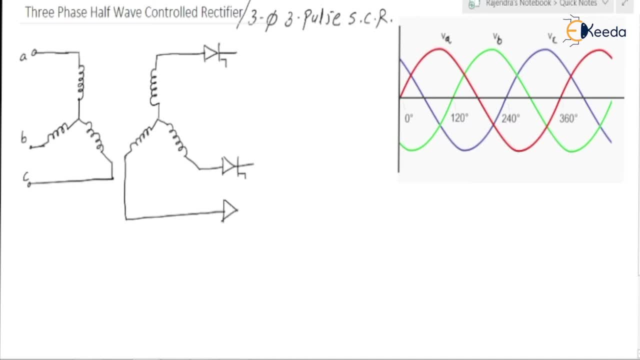 Next, let us consider the SCRs as T1,, T2, and T3.. The T1, T2, and T3.. One is the T1, T2, and one is the T3.. Okay, Next, here we will be having the load. 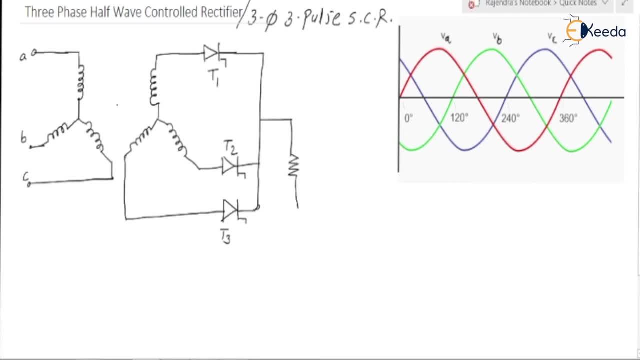 Let us first consider the load is purely resistive. Okay, Later on we are going to discuss the operation for REL load as well. So this is the circuit diagram, The circuit diagram we are having Right for T phase of the controlled. 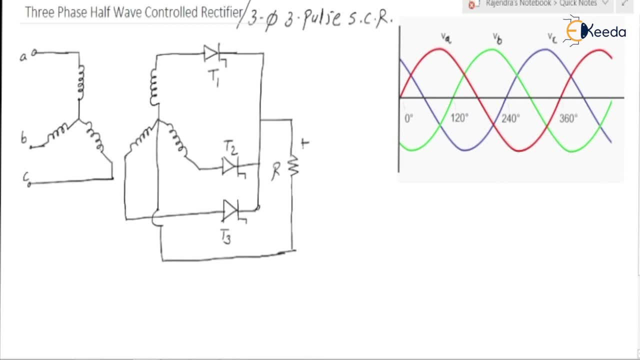 resistors: okay, R to V0 voltage across the load: I0 current to the load. okay, So it is like a neutral point, right? Next, let us consider this voltage is V8, right, Consider? let us consider. 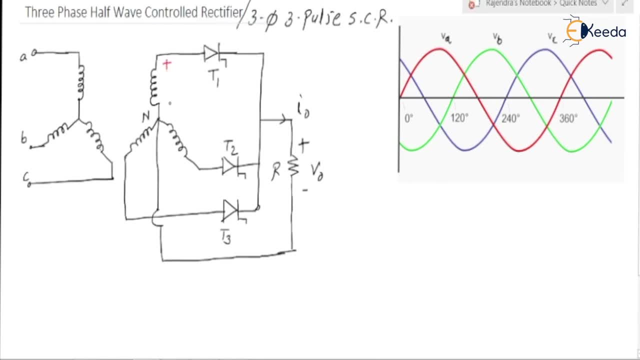 this voltage is V8. right, Let us consider: this voltage is Vb. this voltage is Vb, so here it is the phase A. we are having phase B- the supply, and here it is the phase C supply. okay, So if you check, this is the circuit diagram. 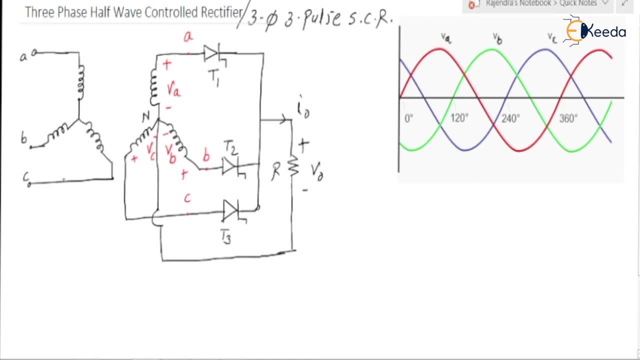 where, okay, The primary winding of the transformer, three-phase transformer: right The primary winding. it may be connected in star or it may be connected in delta, But be careful, the secondary should be always connected in star. only because for this circuitry. 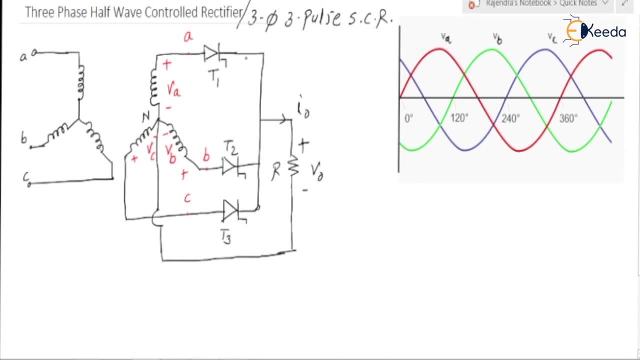 we require three-phase, four-wire supply. okay, So four wires are: yes, this is the first wire, here it is the second wire, here it is the third wire and here it is the four wire. right? So we are having the four wires and 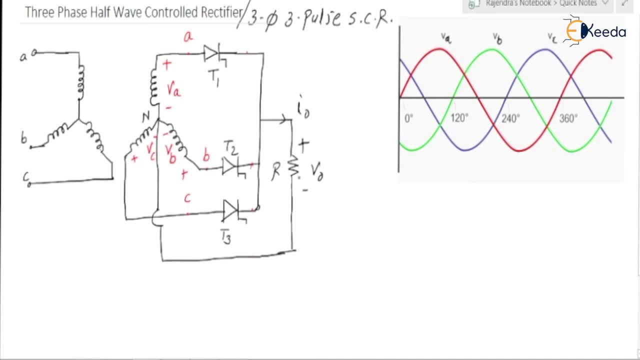 we are having the three-phase supply. okay, Here I have considered the load is purely resistive. Voltage across load is V0, current flow through the load is I0,. okay, And this is the rectifier circuitry. okay, So input is: 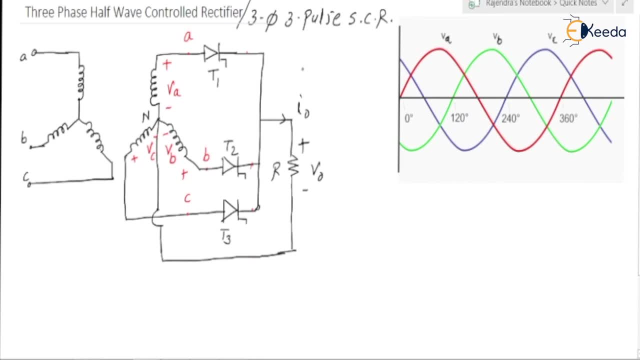 the AC right And output expected is the DC. okay, Now, if you check the waveform of the supply voltage right, This is the waveform of the supply voltage Vs. okay, It consists of the three-phase balanced supply, that is, the Va, Vb, Vc. 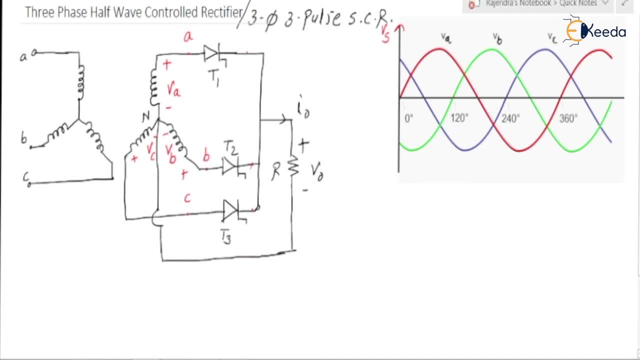 these are the three-phase balanced supply: Va, Vb, Vc. okay, What do you mean by the three-phase balanced supply? Yes, the three-phase supply is said to be balanced If there exists phase displacement of 120 degree right. 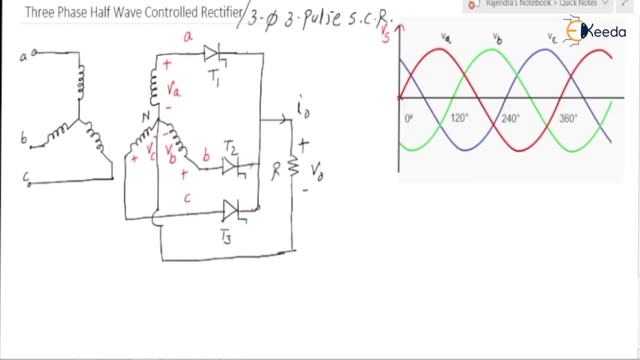 If there exists a phase displacement of 120 degree right, So between just all the three-phase voltages. The second requirement is the frequency of all the three-phase voltages as well as line voltages. it should be same, okay. Next third requirement: the RMS value. 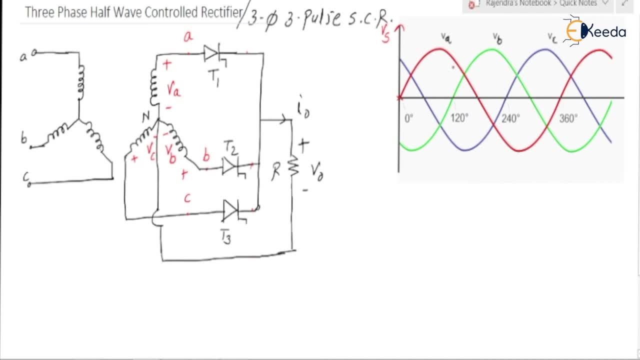 and the peak value of the phase voltages and the line voltages as well as line voltages. right, Should be same, okay, So here we are having the phase voltages Va, Vb, Vc. okay, If you check this. 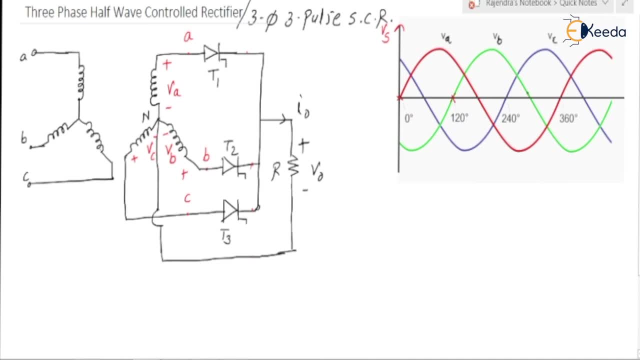 angle is 0 degree right, This angle is 120 degree right And this angle is 240 degree. okay, So here, yes, if you check Vb, can we say that Vb is starting after 120 degree, right? So Vb is lagging to. 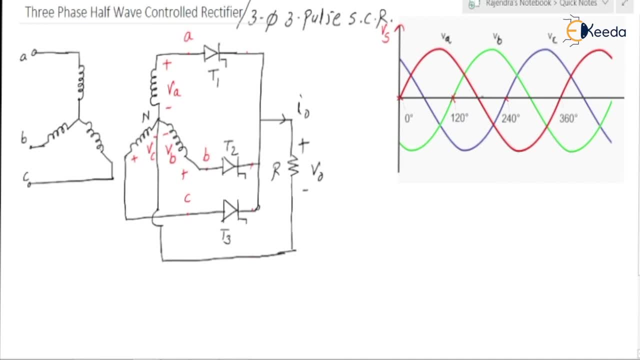 Va by angle 120 degree. yes, Vc is lagging to Va by angle 240 degree, as well, as Vc is lagging to Vb by angle 120 degree. okay, So here we are having the three-phase balanced supply, If you. 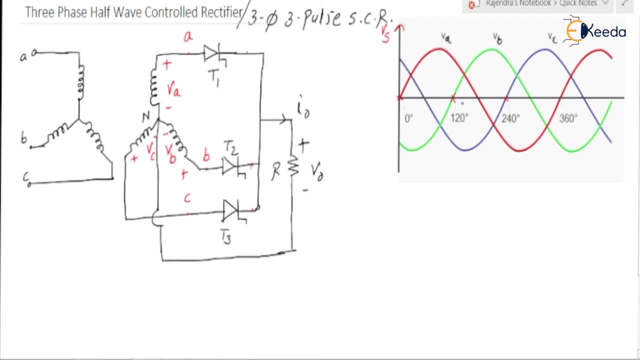 check the peak value of Va, Vb, Vc. it is the same. okay. Now the question is why we have drawn the only phase voltages as the supply voltage in this case, okay. Why we have not drawn the line voltages, okay. So let us discuss. 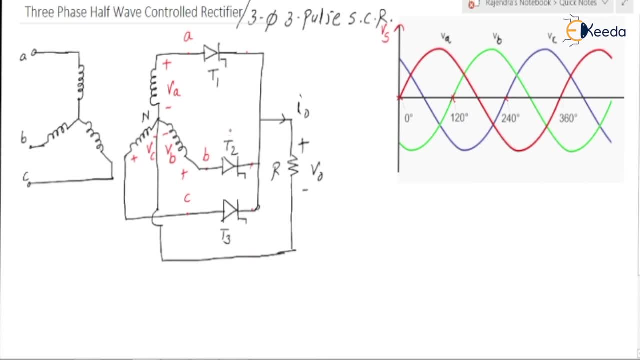 Here in the circuitry. yes, we are having the three thyristors, okay, And, as I said, yes, at a time, only one thyristor will be in the on state. okay, So in the circuit operation. 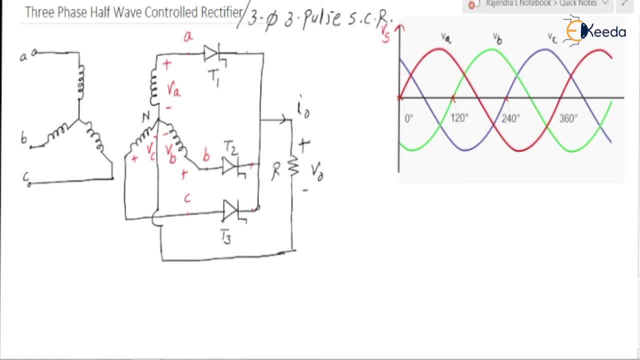 yes, we are having the three thyristors T1, T2, T3. At a time. only one thyristor will be in the on state, okay, And remaining two will be in the off state okay. So suppose if thyristor T1 is in the on. 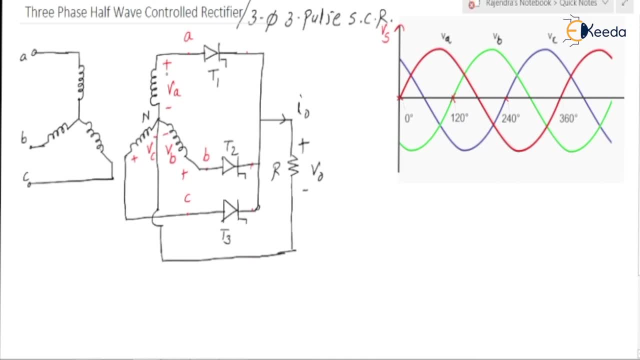 state okay. So how the current will be flowing. Yes, current will flow from Va, yes, load, Va, T1, load and again back to the neutral right. So when T1 is in the on state, current will. 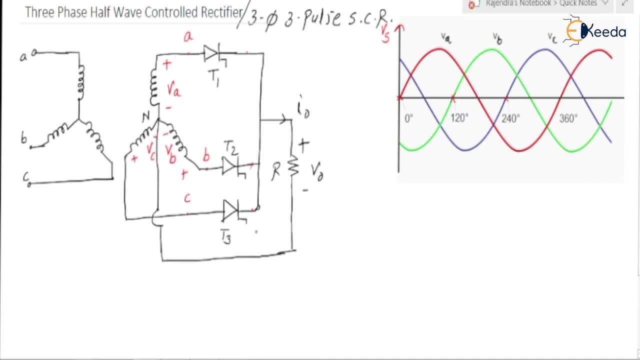 be flowing like: yes, Va, T1,, load and again back to the neutral point. okay, So what is the V0?? V0 will be same as that of the Va. okay, So here can we write it as: 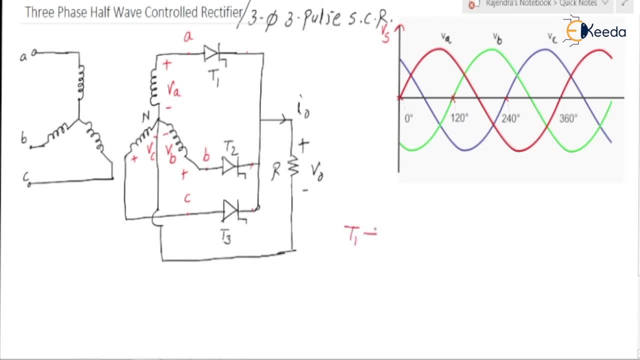 when T1 is in the on state right. So when T1, is in the on state, at that time, yes, what is the V0?? V0 is equal to Va right. Similarly, when T2 is in the on state when. 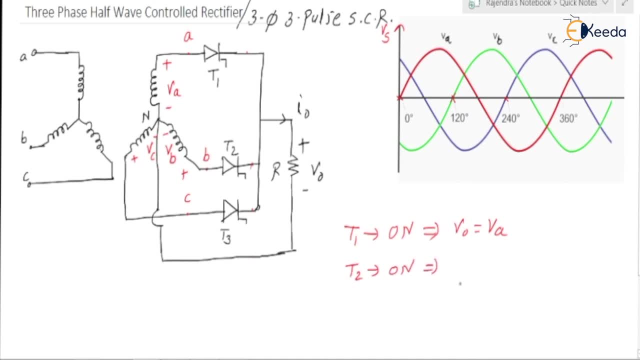 T2 is in a on state at that time. what is the V0?? Yes, V0 is equal to. if you check, T2 is in the on state. okay, So current will be flowing from Vb, T2, load and again. 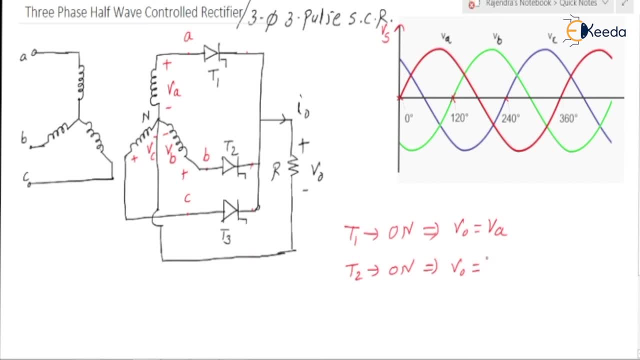 back to the Vb. okay, So V0 is equal to Vb. okay, V0 is equal to Vb. Similarly, when T3 is in a on state, when T3 is in a on state, yes, at that time, yes. 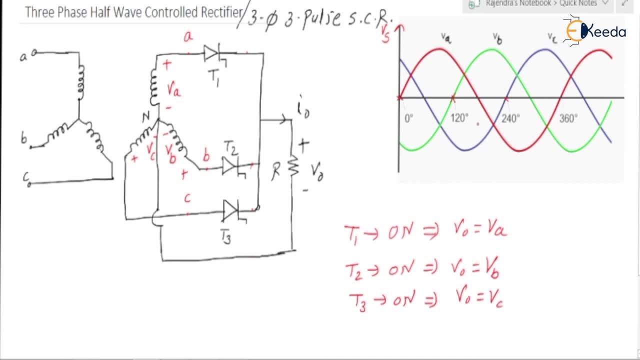 the voltage V0 is equal to Vc right. So, as I said, at that time only one thyristor will be in the on state. So one thyristor when it is in the on state, at that time the voltage that will be appearing across. 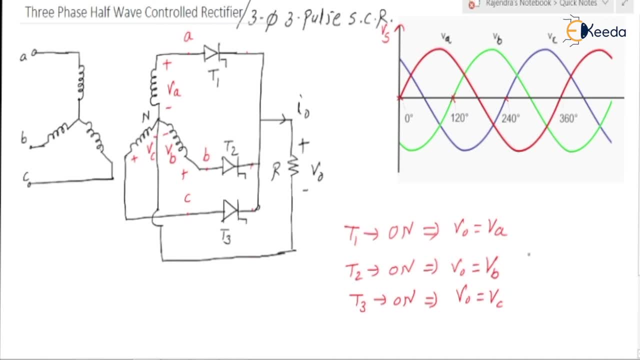 the load is nothing but either Va, Vb or Vc. okay, So some part of Va, Va is the line phase voltage, Vb is also phase voltage, Vc is also phase voltage, right? So here we are having the star. 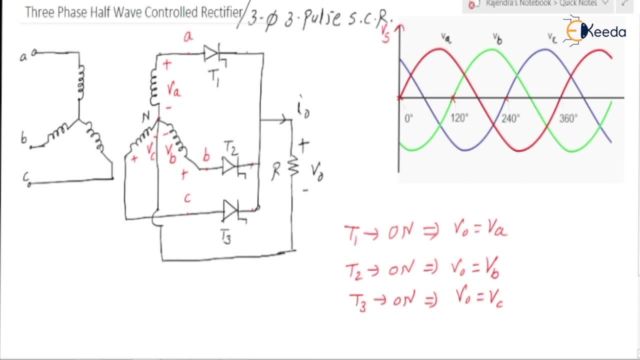 connected supply right. And, as we know, yes, potential difference between point A and the neutral point is nothing but the phase voltage, that is, the Va right. The potential difference between point B and the neutral is the phase voltage- Vb right. 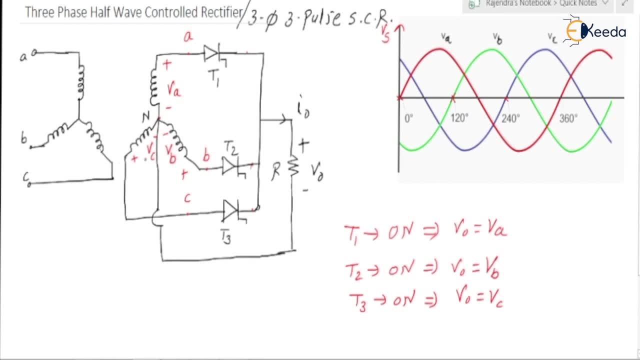 Potential difference between point C and the neutral point is nothing but the phase voltage Vc. okay, So that is why, as the output voltage will be equal to, yes, some portion, right, Equal to some portion of the respective phase voltage, okay, So therefore. 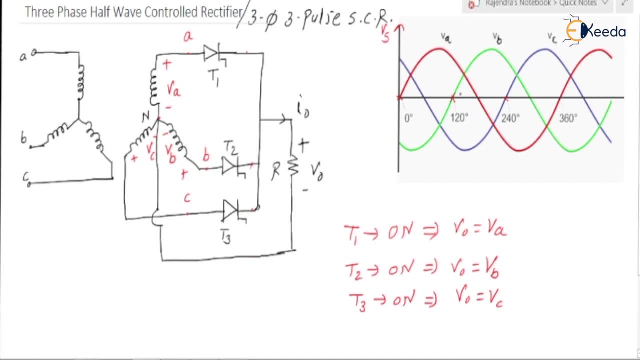 we have considered the Vs, that is, the supply voltage, is nothing but the phase voltage, phase voltage, waveform. okay now, yes, in the circuit operation we are going to apply the balanced three phase supply to the primary winding of the transformer right. so balance the three phase. 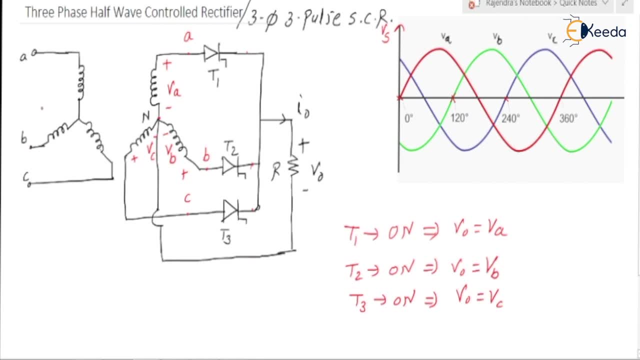 supply we are going to apply here. okay, after that, what will be happening? yes, transformer is a circuitry, yes, that transfers the electrical energy from one electrical circuit to the another electrical circuit without any electrical connection between them. okay, so here, if the balancer supply is appearing at the primary winding, definitely, whatever the supply, that 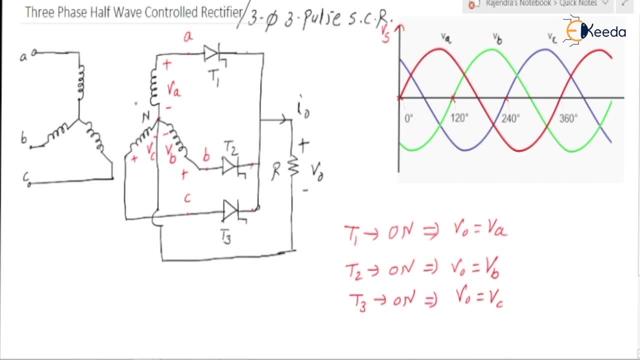 will be transferred to the secondary winding? definitely it will be the balanced only, okay. so that's why we are having va, vb and vc. that is, the balancer supply. is this clear, okay? so this is the prerequisite, right, or the very basics, for the understanding of three phase half wave.